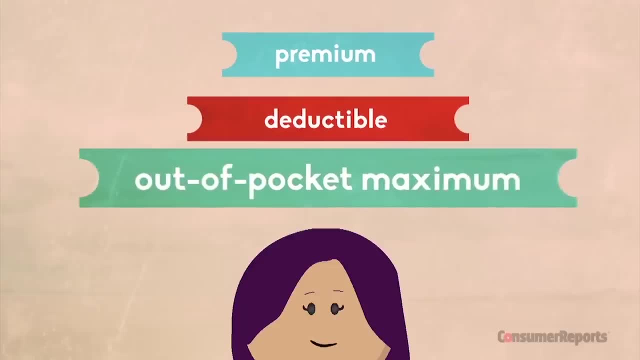 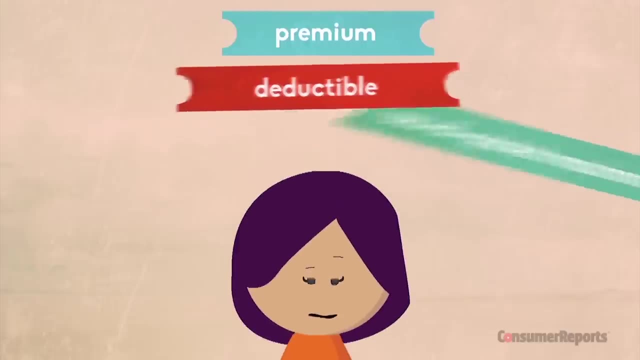 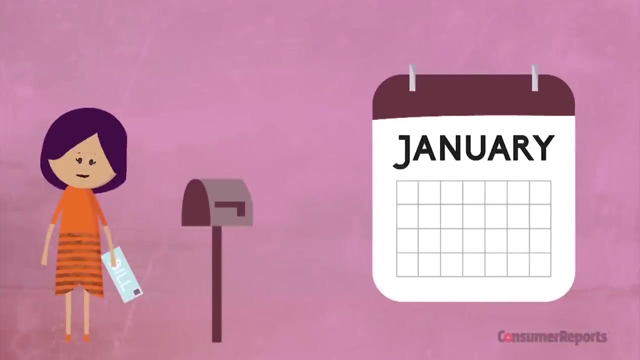 Premiums, deductibles and out-of-pocket maximum. It may sound complicated, but stay with us, It's not as hard to understand as you think. First, premiums: Think of your insurance as a monthly membership. Every month you pay the same amount in order to be a member. That amount is your premium. With your premium, say $200 a month, you get some preventive care for free. This includes care like vaccines, medical costs and screening for diabetes and cholesterol and breast cancer. This care is covered by your premium. but what if you need more than just preventive care, If you need a health service beyond preventive care? 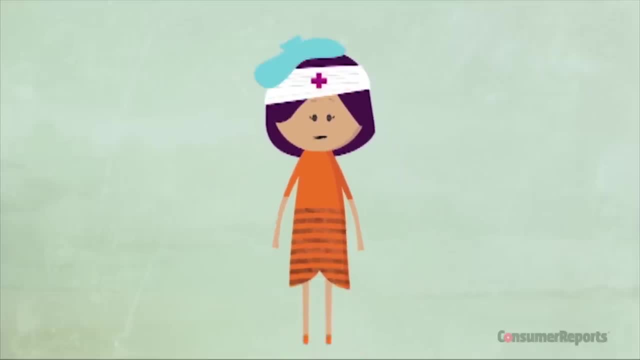 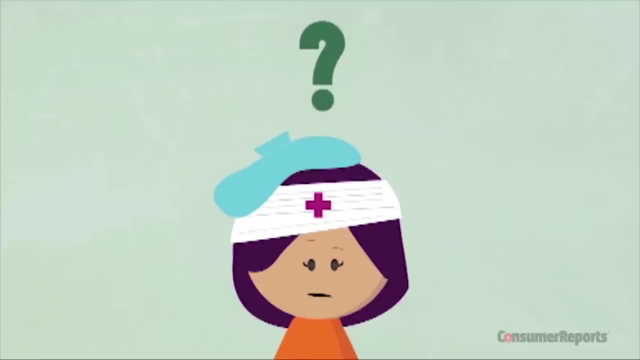 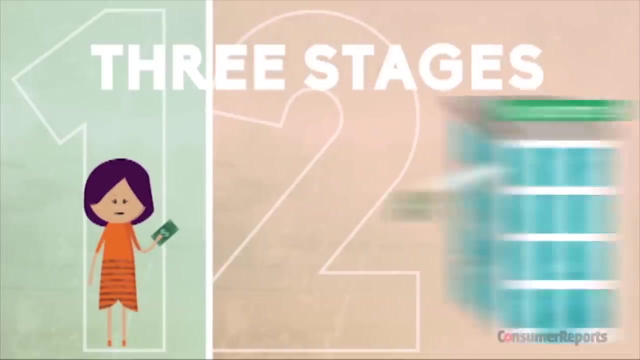 illnesses, a broken leg, emergency room visits- you usually need to pay extra. How much? Well, that changes over time. There are three main stages: First you pay, Then you pay for your insurance, Then your insurance pays some and you pay some. 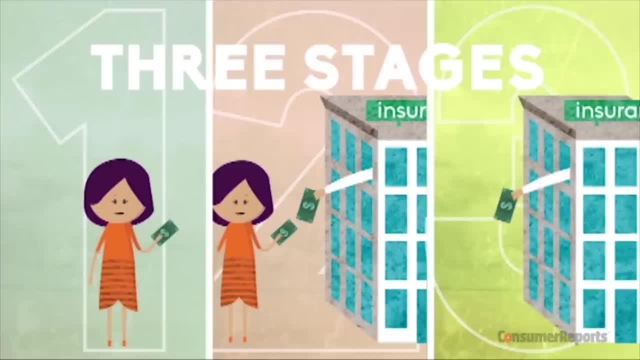 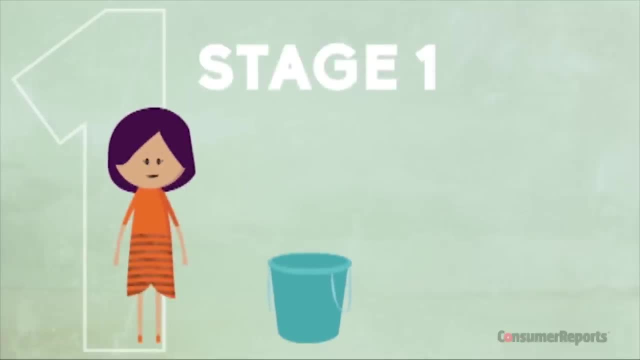 And finally, your insurance pays everything. So how does this work? In the first stage, at the beginning of the year, you pay for most of your health care until you reach your deductible. Remember that word: Deductible. A deductible is the amount of money you have to pay for your care before the insurance. company will share the costs. So let's say your deductible is $500. That means almost every time you get health services you will pay for all those services until you've paid a total of $500. It's like you're filling up a bucket. 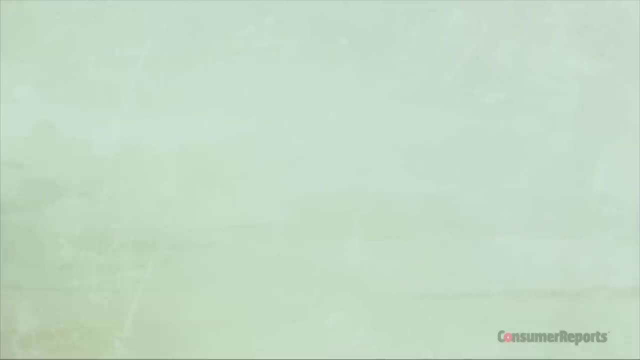 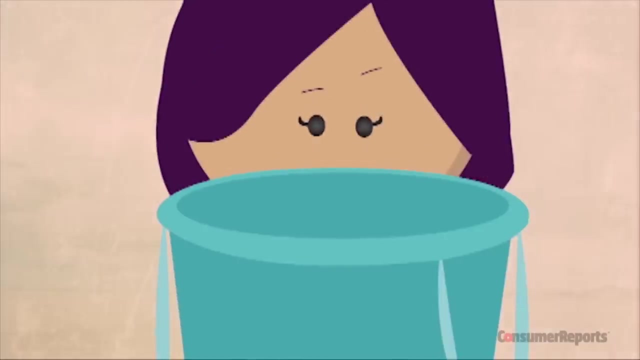 Once you add enough to that bucket so that you pay your whole deductible, then everything changes. Then you enter into the second stage. Now. every time you get health services, your insurance company will share the cost of those services. How much, That depends on your plan. 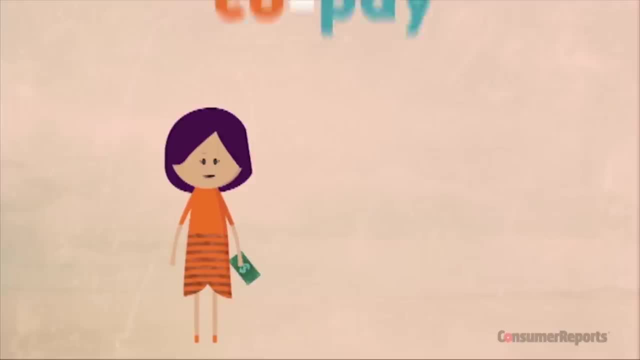 Usually you pay part of the cost- fees, called co-pays or co-insurance- and your insurance pays the rest. But the second stage doesn't go on forever. If you reach a certain amount, you won't have to pay for any services. Remember that bucket. Every time you fill it with co-pays and co-insurance, your insurance company is keeping track. If you fill that bucket up to the top, everything changes again. You enter stage three. From this point on, your insurance company pays everything for the rest of the year. 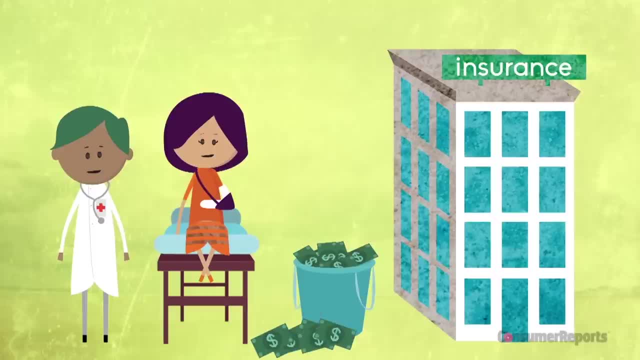 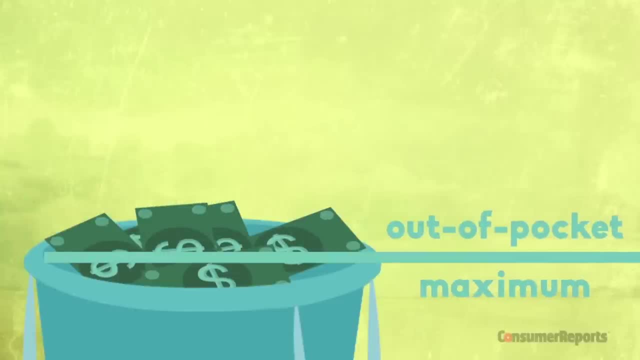 That's right. Every dollar of your health services paid by your insurance company. So what's at the top of that bucket? It's called your out-of-pocket maximum. This is the most money you will pay for your health care over an entire year. So let's say your out-of-pocket maximum is $2,000.. After you pay your $500 deductible And If you pay an additional $1,500 for various health services, you've hit your out-of-pocket maximum. From then on, you don't pay a penny more for covered health care services.